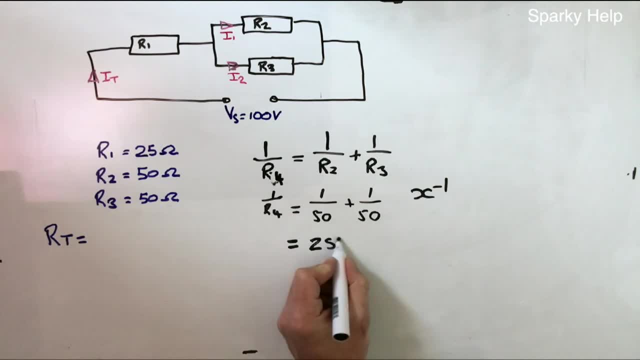 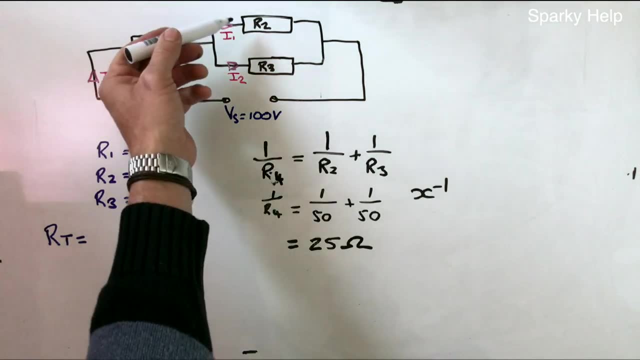 And if you do all of that, it will come to. some of you probably have already noticed it should come to 25 ohms. This happens to be the case because I've chosen it. But when you have the same in parallel, you just take one of them and divide by the number of them. 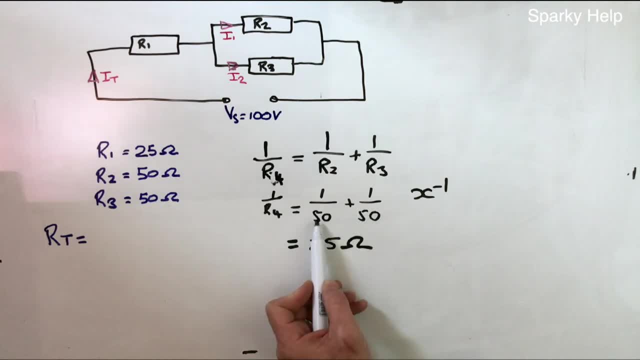 So there's 0 for 50, there are two of them. So 50 divided by 2 is 25.. But again, if we do the x to the minus 1.. So 50 divided by 2 is 25.. But again, if we do the x to the minus 1.. 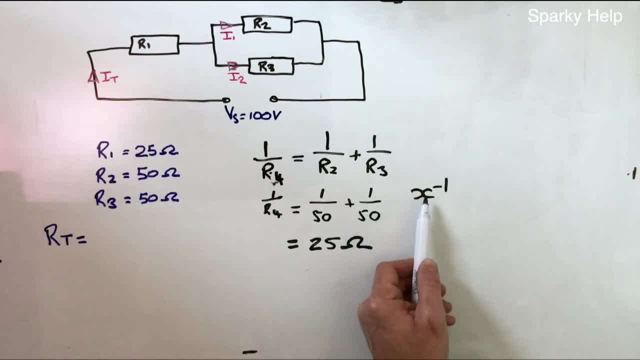 So that's 50, x to the minus 1,, plus 50, x to the minus 1, equals x to the minus 1.. Your answer: that will give you your 25 ohms. That then breaks the circuit down. 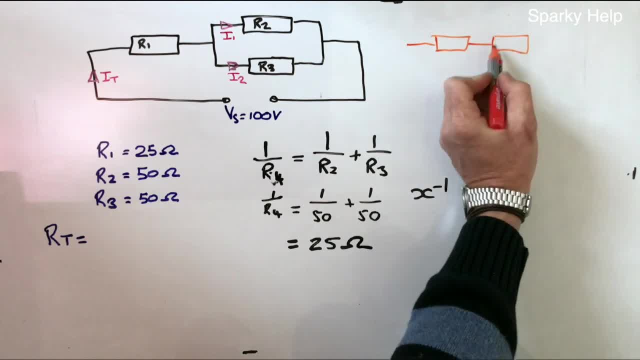 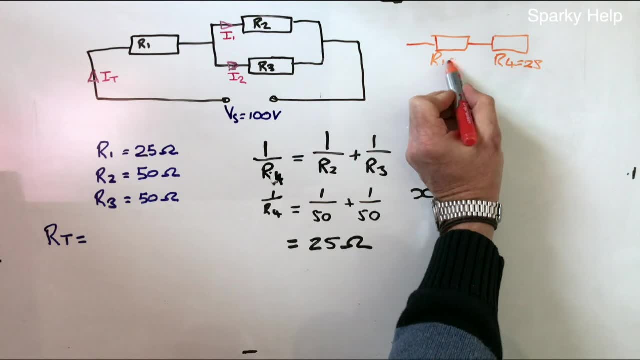 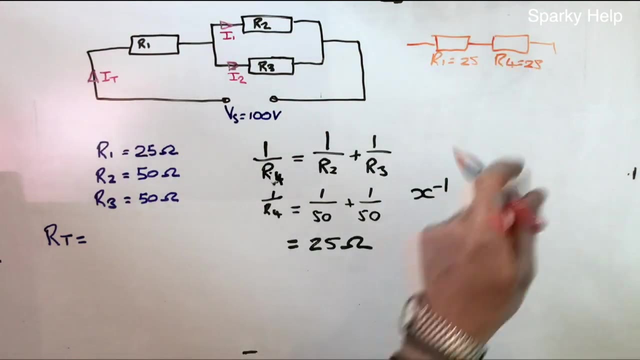 So what we've now got is this: R4, which we now know is 25.. And R1,, which is 25 as well. So we've now broken this circuit down into just a basic series circuit And we can now find RT. 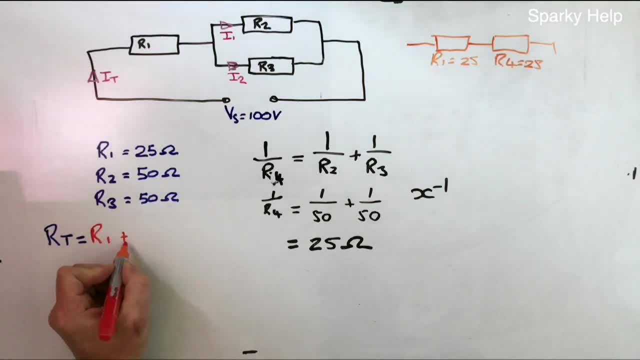 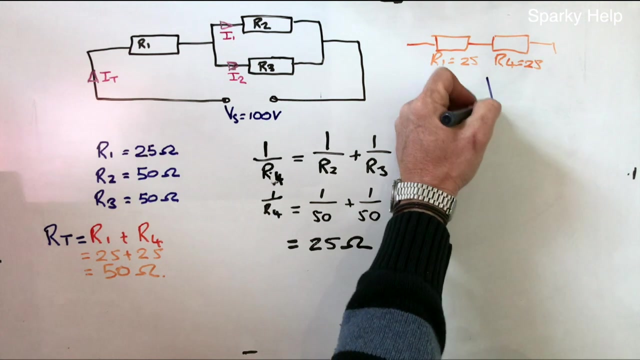 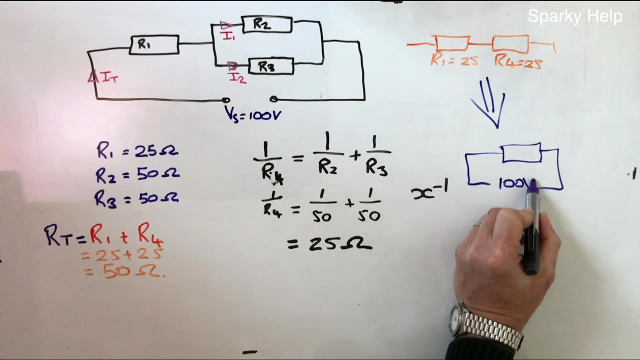 So RT becomes R1 plus R4. And R4 is this combination here, If we put these figures in, So RT for that entire circuit Is 50 ohms And that can again be drawn simplified into that entire circuit As so. 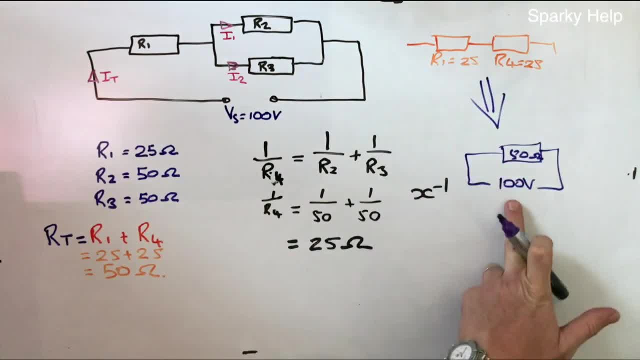 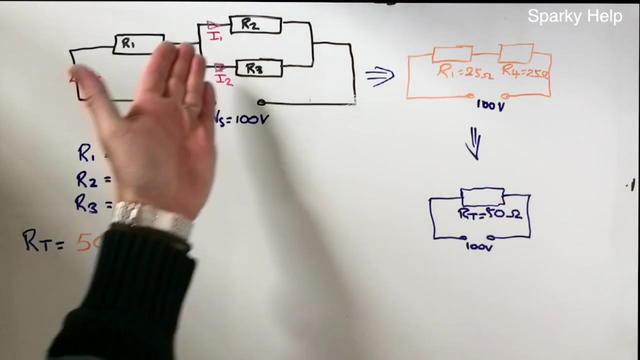 So we've started off as a series parallel, Gone to a series down to 1.. These are our three steps we've taken to get to our final answer, RT. OK, now we've made the circuit into three broken down pieces effectively. 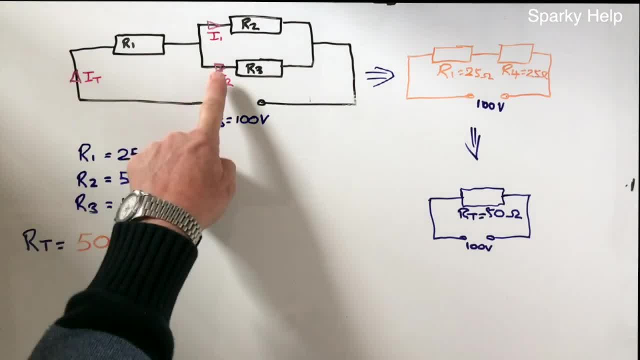 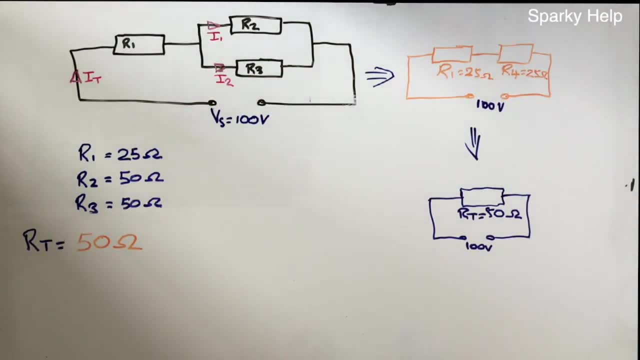 We know RT is 50. What we're now allowed to do is calculate these three currents. This possibly makes it a little bit easier to work these out. We'll start off by working over this one here, Because this is the total of the circuit. 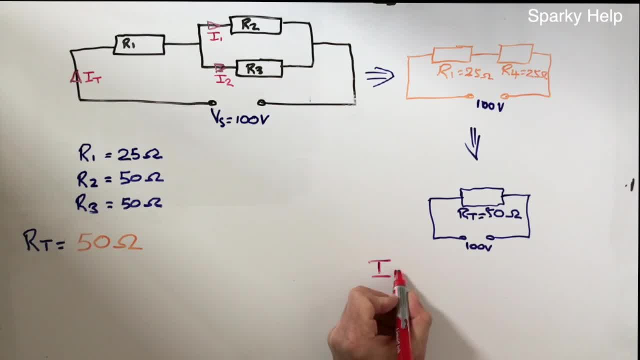 From previous examples. IT is equal to VS Divided by RT, Which is Ohm's law. So if we put these figures in 100.. Because this is the total Divided by RT, Which is 50.. Maths is not difficult. 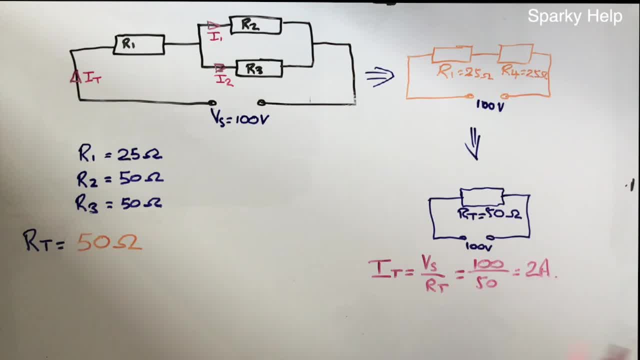 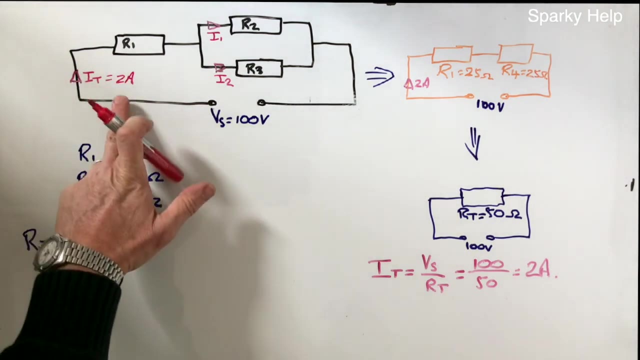 It's the principle we need to understand. 2 amps. This 2 amps, then, would be the same 2 amps that flows around in this circuit here. More importantly, it's this 2 amps over here, This 2 amps, then. 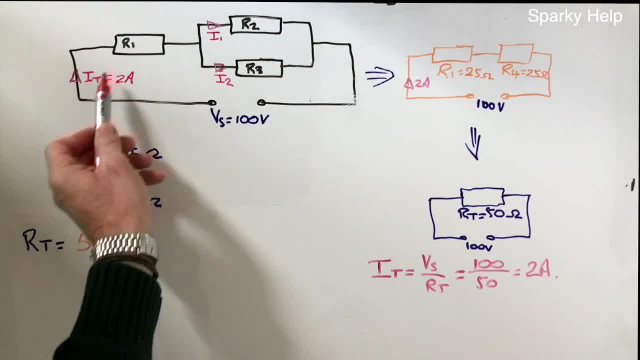 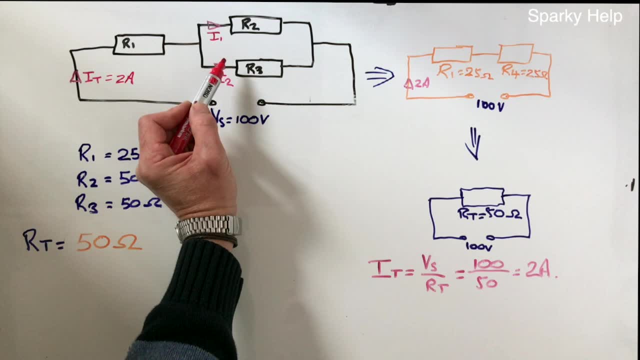 Flows out Must come back. So it's going to 2 amps will pass through the R1.. When it gets to this point here It will split OK And split into I1 and I2. Depending on the value of these resistors. 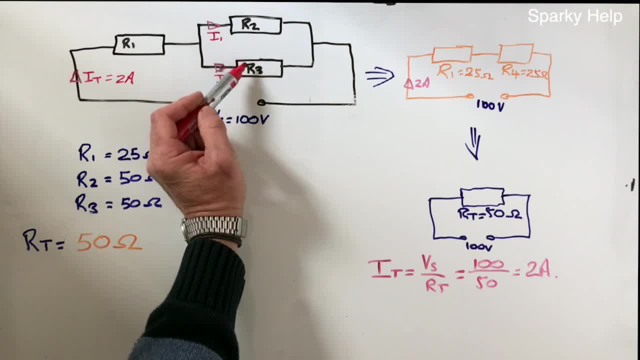 Will determine which current, And how much current, goes each direction. So How do we work that one out? Well, To be honest, There's not much to work out on this one, Because we know These: 2. Are equal. 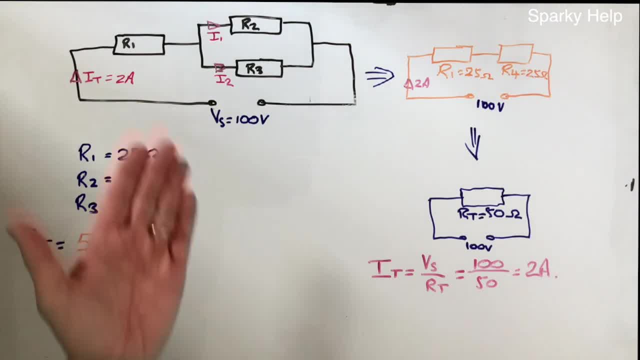 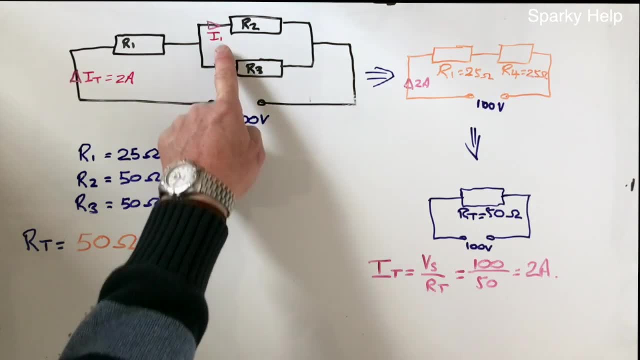 They're both 50.. So if they're equal, The current has to split Evenly. Therefore it will divide by 2.. So I already know, And hopefully you've all recognised it: There'll be 1 amp pass through each one. 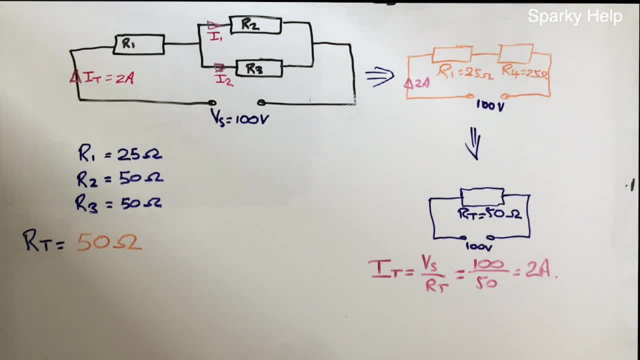 But if we needed to work it out, We'd have to do a calculation, So we'd have to work out I1.. Let's work that one out first. Well, the formal use for that Is Ohm's law, So that would be. 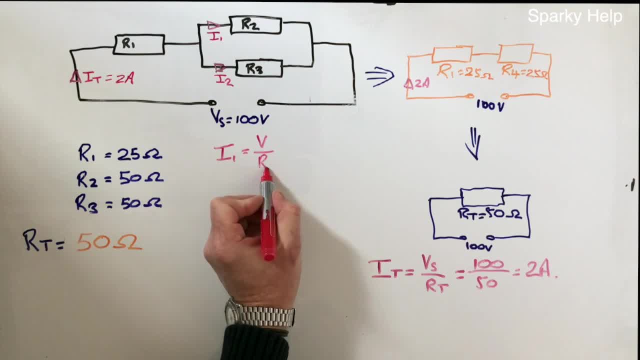 V Divided by R, The difference being. Now, though, We want to calculate That current. So this is our formula. It's Ohm's law, But it's. which voltage Do we apply? Because what it isn't? 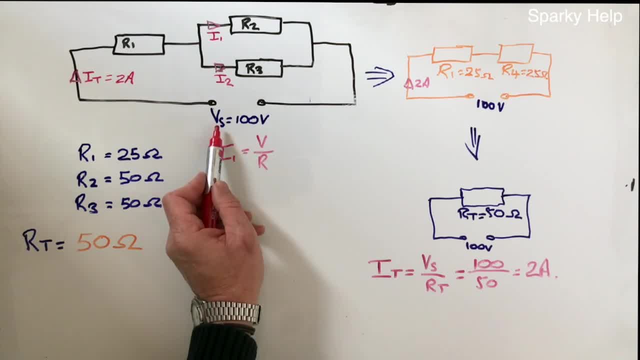 It isn't Vs, Because Vs Is not across That resistor. And that's what we're trying to find: The current flying through That resistor there. So in order to work that one out, We've got to find The volt drop. 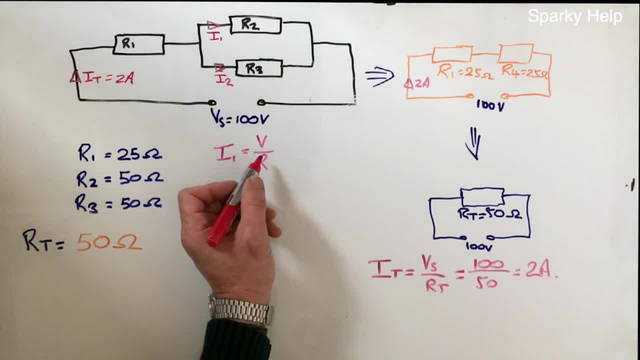 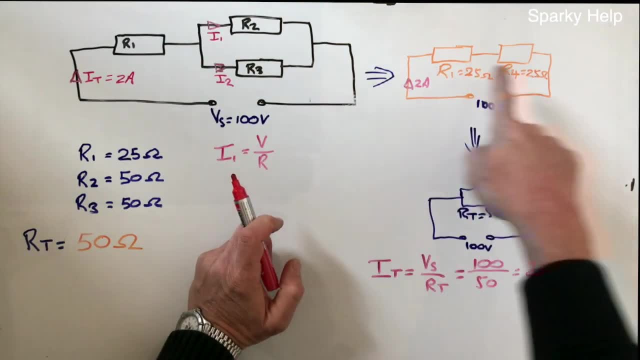 That resistor And that's what we're trying to find: The current Flying through That resistor there. So in order to work that one out, We've got to find The volt drop Across This resistor, And that's easier. 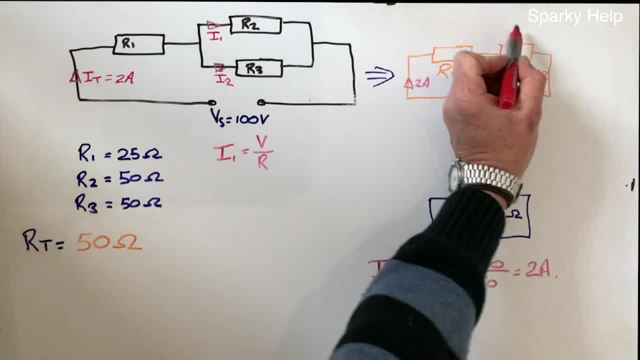 To work out From over here. So to work this voltage out, Let's call it V1.. Just a really confused method. So to work out that voltage there, V1. Which is what we're trying to work out. It is. 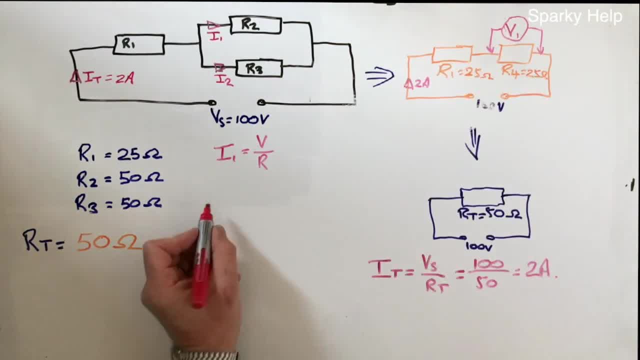 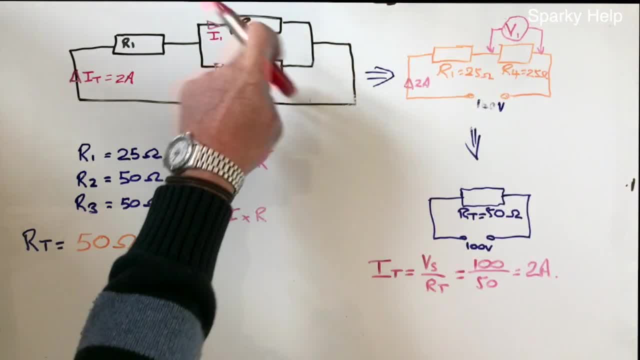 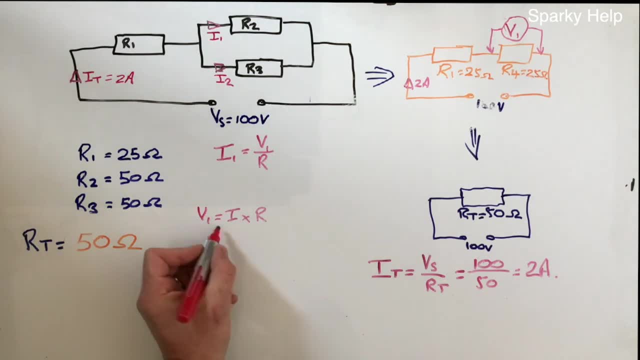 To find that voltage there, Because this one Is all of that Okay And we know from a parallel circuit that voltage in a parallel circuit Will stay the same. So to work this one out Is to би the power that passes through that. 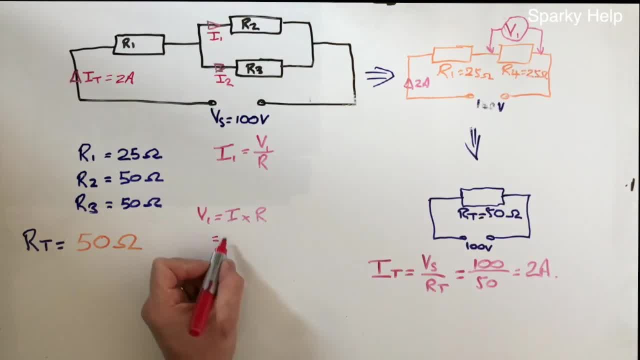 So this one here is 2 amps, Cause it's a combination of the two. So it becomes- I'd T from over here Times R4. And R4, we know, is 25.. So that becomes 2 times 25, 50 volts. So the numbers now are: 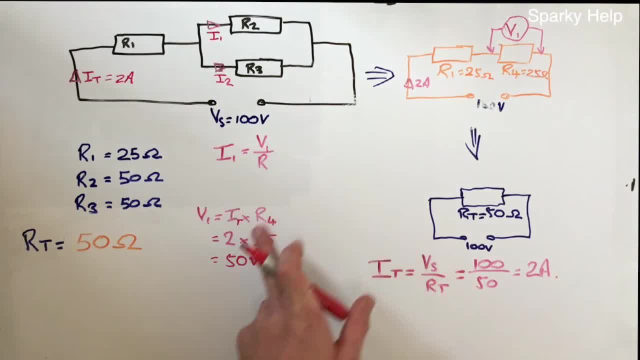 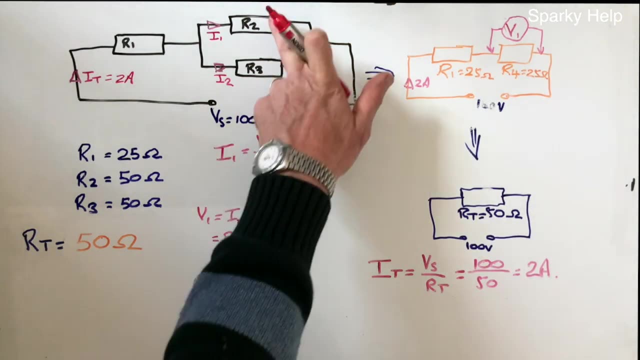 relatively simple, So that becomes V1.. That's what V1 will be. And then you divide by R. Well, there's actually 1,, 2, 3, 4, 5 different R's on here, But because we want to find the 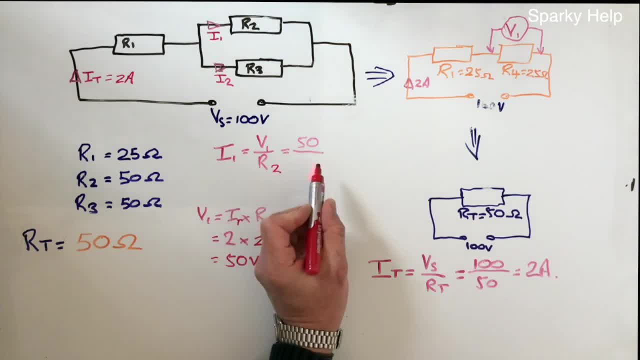 current through that one. it's R2.. So that becomes R2, which is 50.. So 50 divided by 50 is 1 amp. That's our current there. This one can be done exactly the same way if you needed to calculate it, because it would be. I2 is equal. 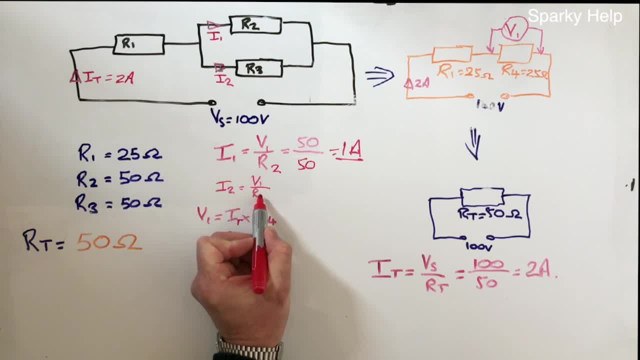 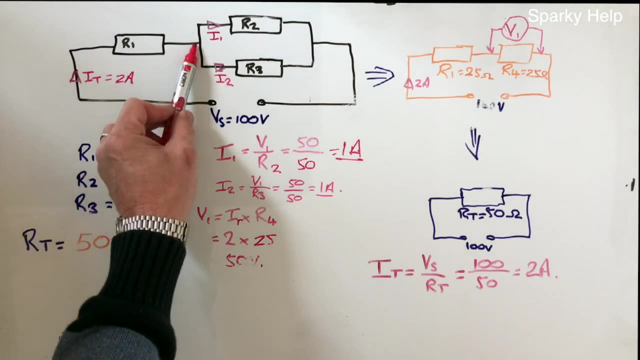 V1,, but this time divided by R3.. So V1, because it's the same thing, becomes 50 again, And it's divided by 50. And that is also 1 amp. That then means this: 2 amps will come up. 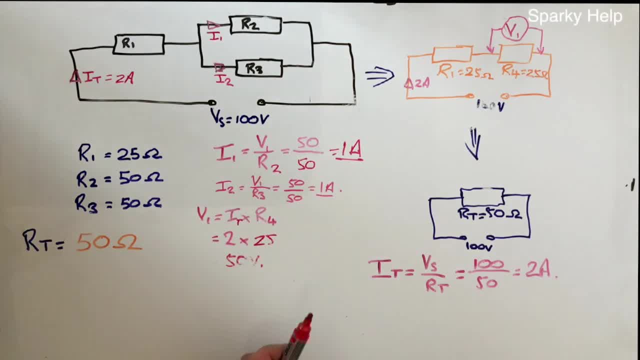 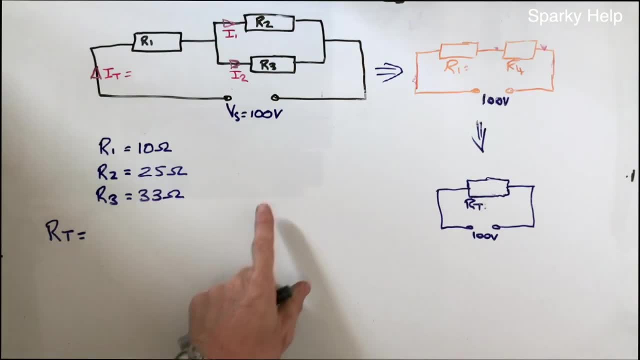 It will split evenly. 1 amp goes through that one, 1 amp goes through that one. And there's your answers to those things there. Okay, let's try it again with a different answer. Set of values, More realistic, I suppose, in the sense that it's harder to work out. 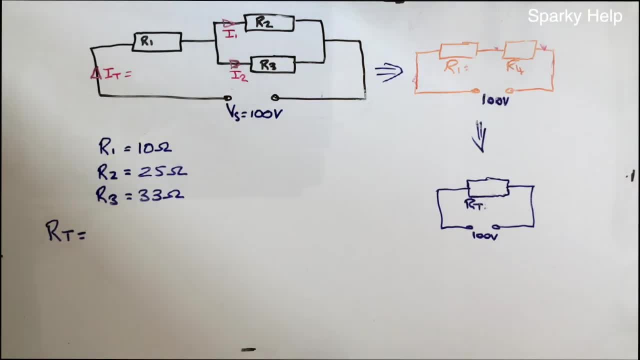 10, 25, 33 for that point there. So, as before, we need to calculate the parallel part first. So we'll call that R4.. And remember, this is parallel, So it's 1 over R4 plus 1 over R2. 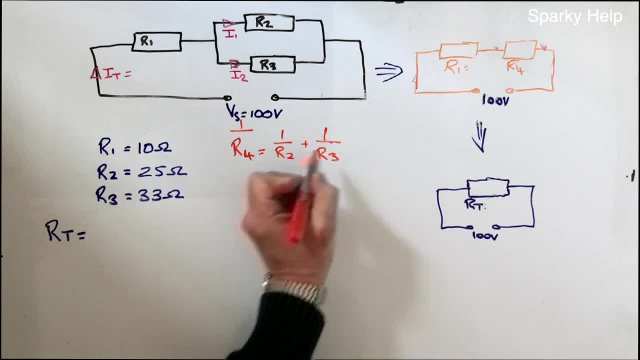 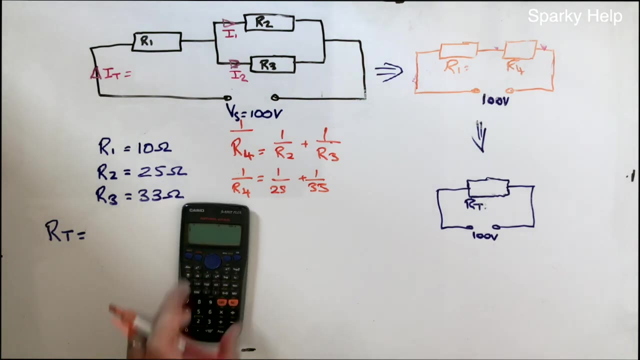 plus 1 over R3.. We put that into our calculators. Ultimately, we'll be looking at 1 over 25 plus 1 over 33.. And remember, it's 1 over as well. for that, This is where we can use our calculator. 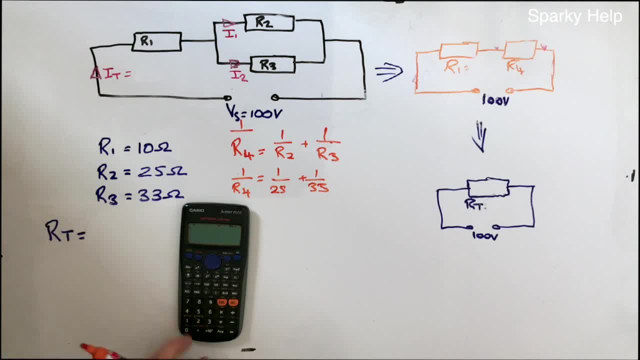 And remember, the button we're going to use is the x of minus 1.. 25x minus 1 plus 33x minus 1 equals Okay, This sets fractions, most calculators. So to do that now we must do x to the minus 1. 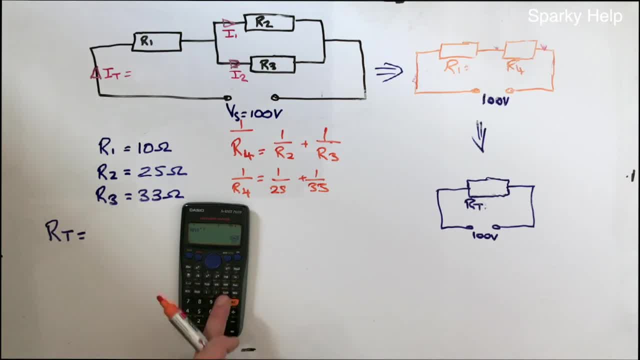 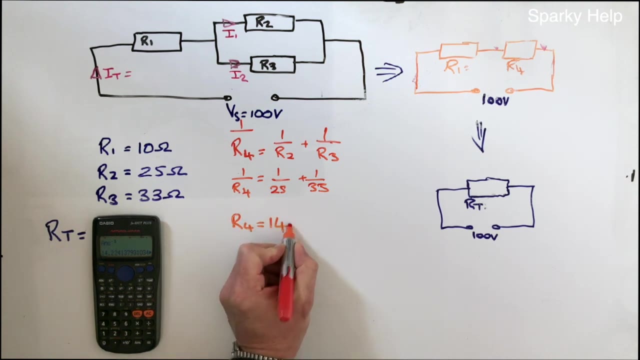 your answer. So x to the minus 1. again, Press equals Comes out as a fraction. Let's do the std. It becomes out as a 14.22. Round, 14.22.. Oops, Okay, That becomes our 4.. 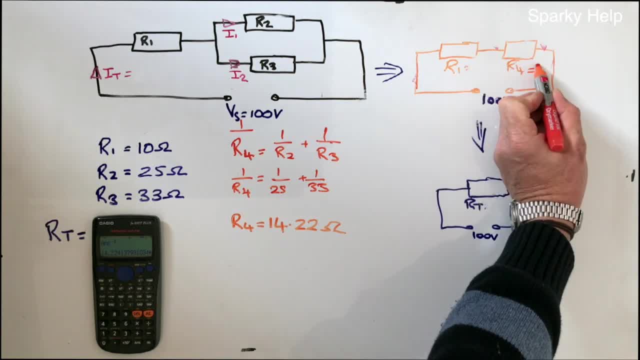 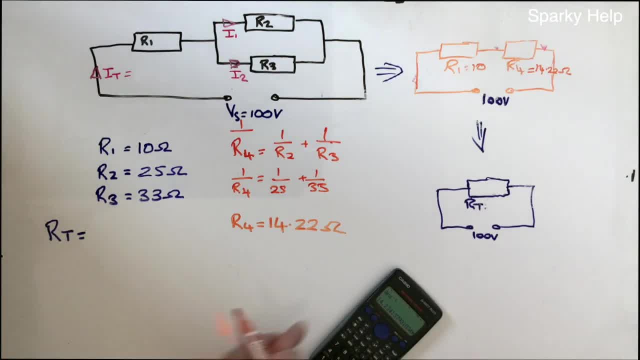 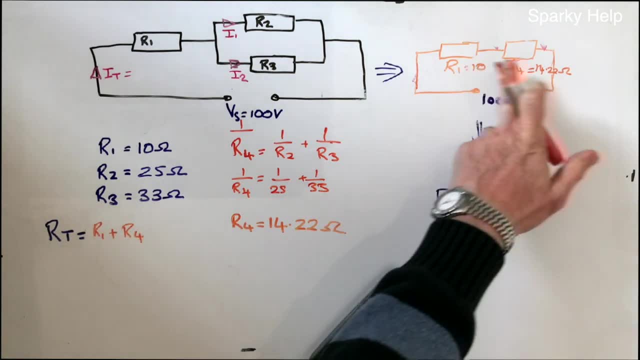 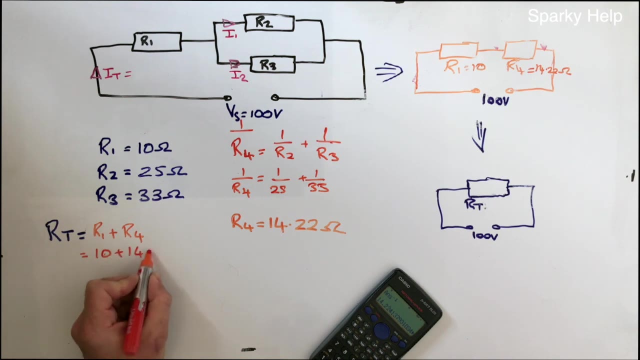 So we can now work out our t. Our t becomes our 1 plus our 4.. Because we're now looking at the series part. If we put these figures in 10 plus 14.22.. So we now know what's going to happen. 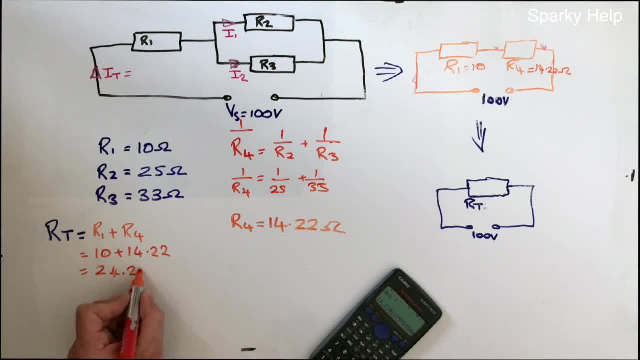 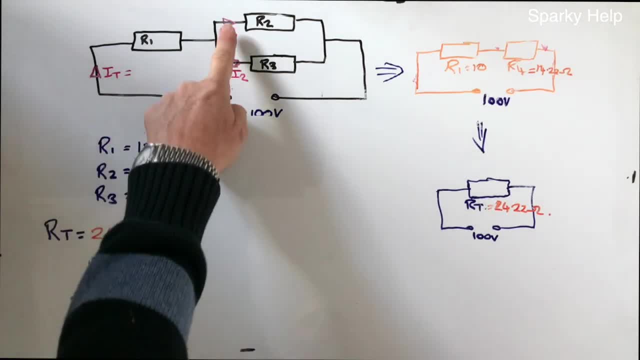 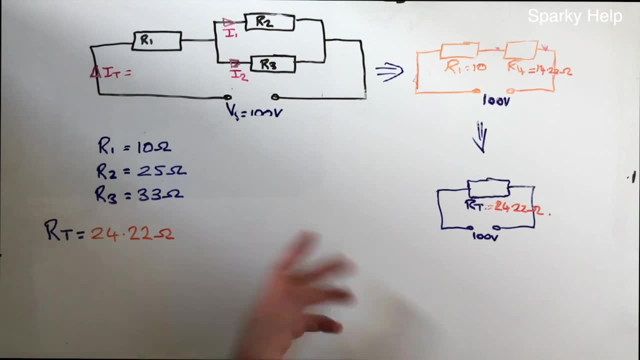 Okay, So work out the currents, then We're going to work out my t over here. 1 and I2, as before. So let's start with IT. this is a nice, simple one, because we can just look at this here, Because, remember, IT is here. it's also here because these: 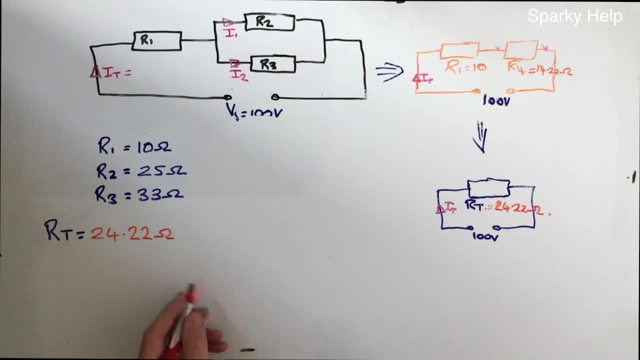 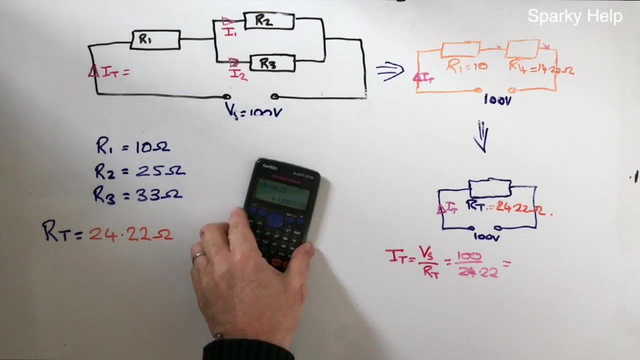 are the same circuits. it's also there so we can work it out here. Therefore, IT using the old law, VS divided by RT, So total, total, and a total So 24,- nearly said the wrong one there- 100 divided by 24.22.. And if we do that into the calculator we will get 4.2.. 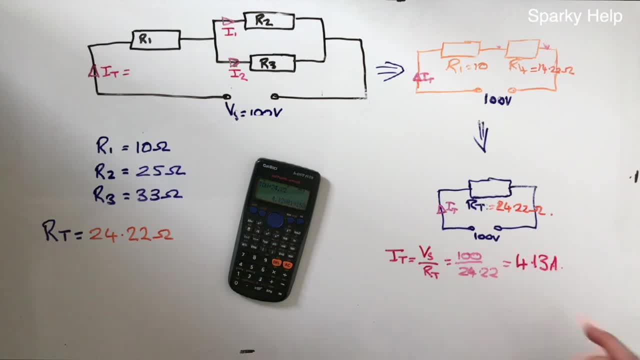 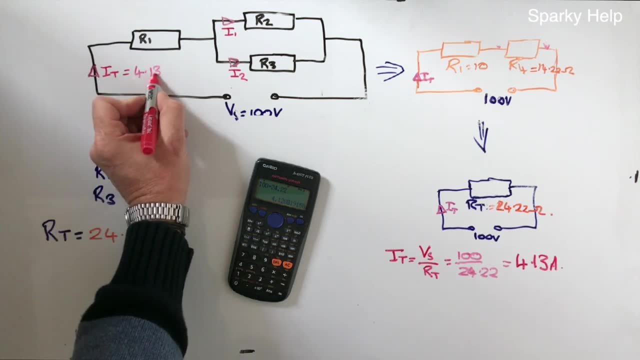 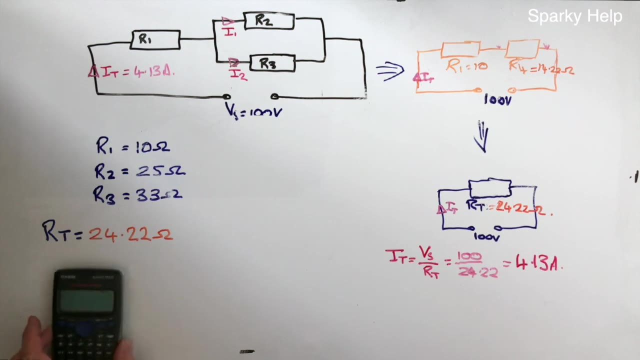 So that, then, is the current flowing through in all these locations. So, IT 4.13 amps, We can now work out I2 and I1.. They are done exactly the same way as we did before. So let's do I1,, which will be owned law, VS So I2,, which will be owned law, VS So I2,. 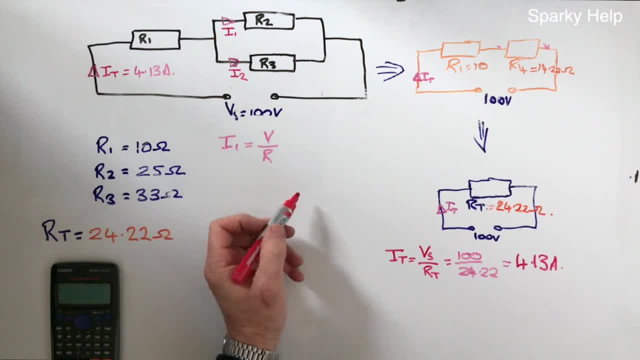 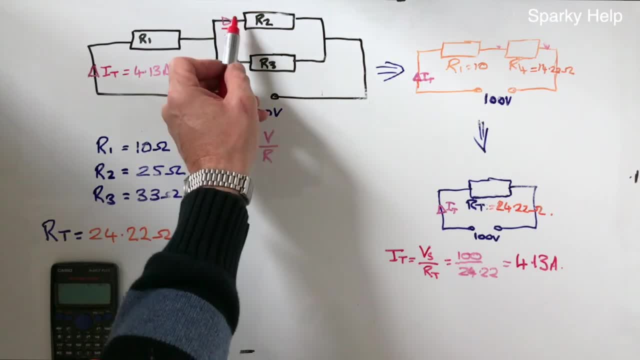 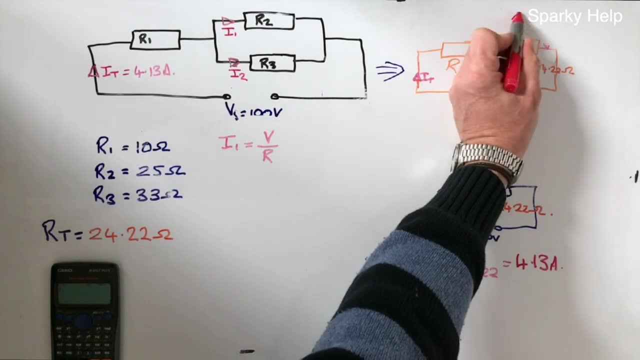 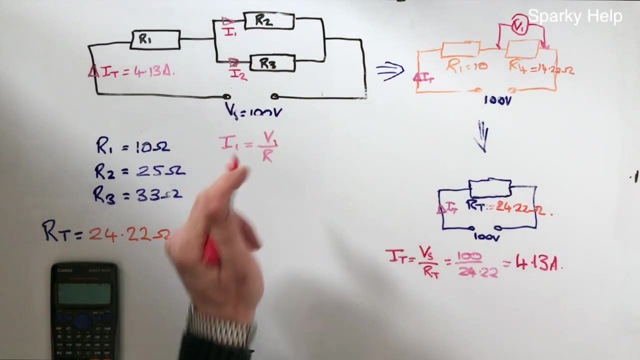 law VS. So it's not VS, remember, because it's not a total we are trying to work out. It has to be the voltage that is in this section of the circuit, So we will call that one V1.. And we're going to find that current there, so it's R2.. So we've got to work out V1,. 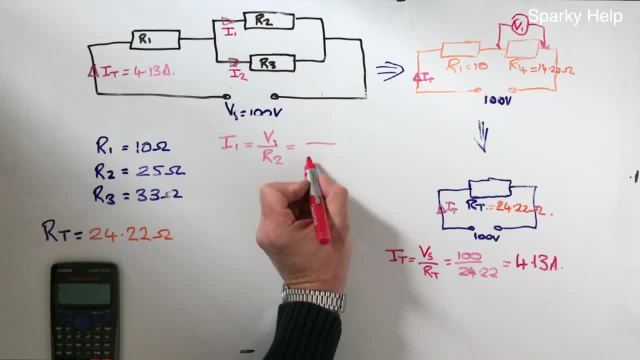 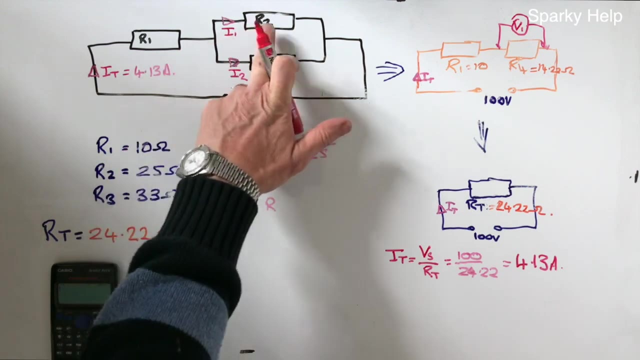 which at the moment we don't know. R2, we do know what that is, that is 25.. So we've got to find V1.. So let's find V1.. V1 is I times R from straightforward Ohm's law, But it's which current? Well, we only know that current. We can't use this.